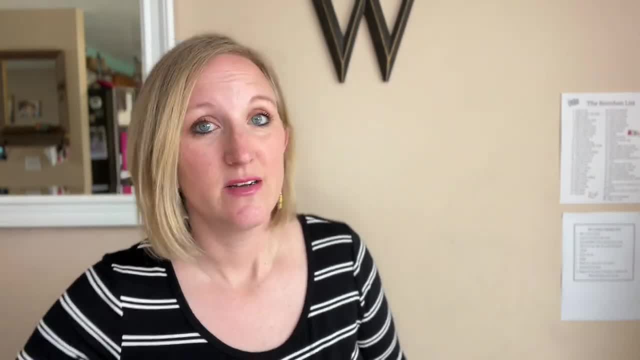 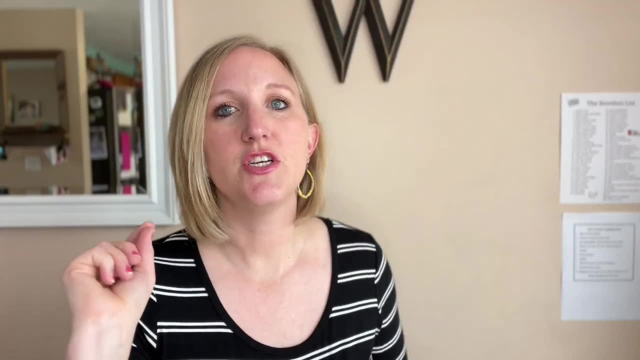 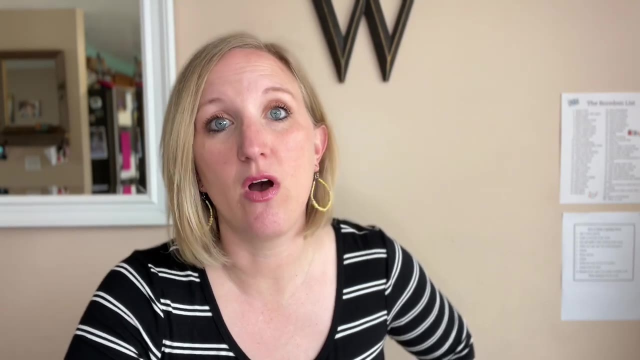 She started with the math curriculum. Math facts that stick, If you know about that. Addition facts that stick. Subtraction facts that stick, Multiplication and division. She started with those and I used those for a long time with my oldest and then one day I got an email from her saying that she is making a full-on math. 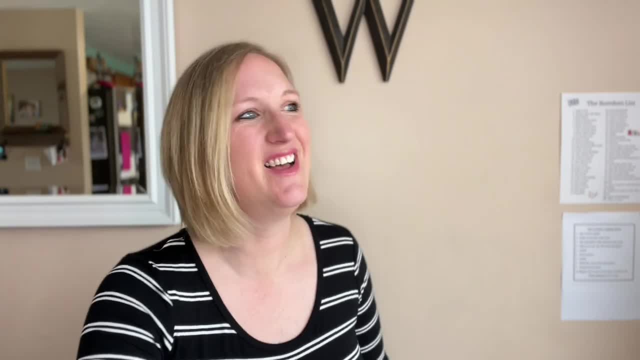 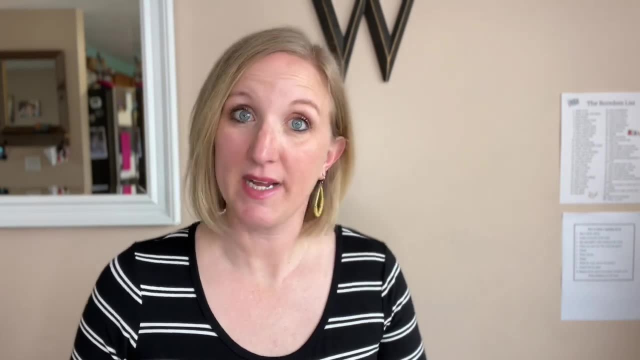 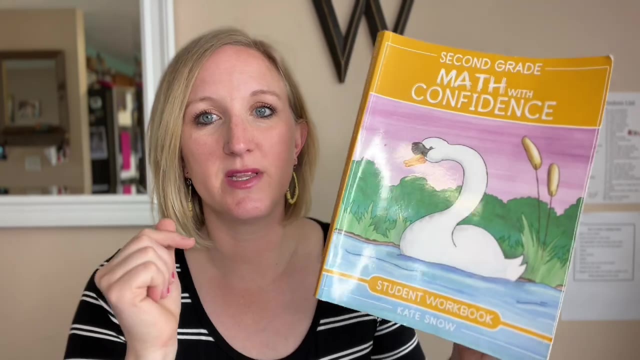 curriculum and I've been following her ever since. So loved first grade. My youngest son loved it as well. Totally wish it would have been around when my kids- older kids- were younger. But maybe you've got kids who are in second grade or going to be in second grade and I highly recommend this. 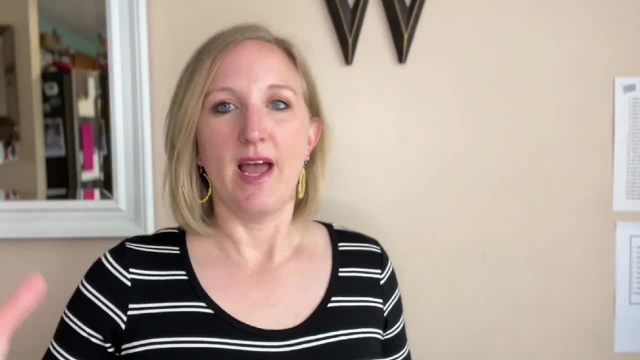 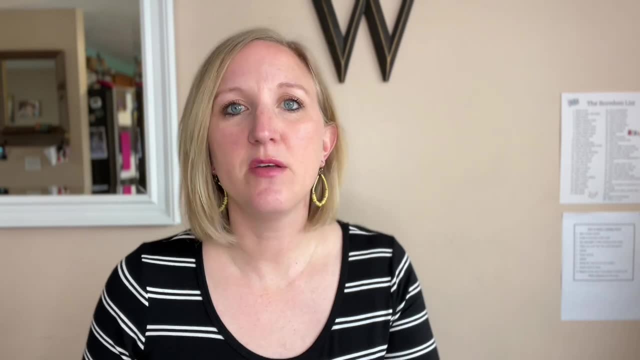 So the good thing about this is it took everything that I really wanted to be in a math curriculum and put it there- It's, it's there. So I wanted something that had a little bit of independent work, because I feel like you kind of in the math curriculum world, you kind of get either or You. 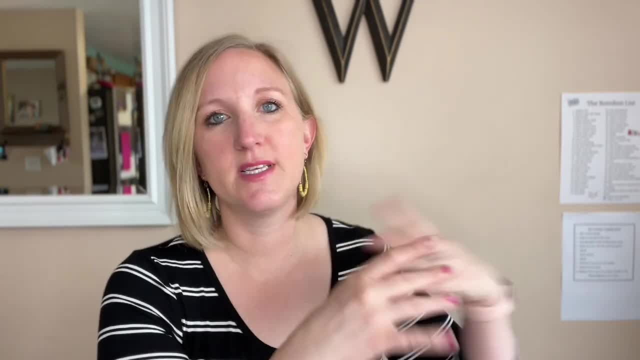 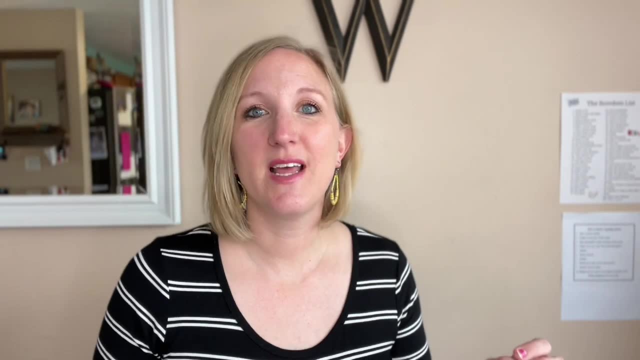 either get a curriculum that is like all hands-on and mom sits with you and plays games and it's great, but then there's like mom has to be there for 30 minutes for math every day. I wanted something could work with my kid. that's another thing is the short lessons, but anyway, sorry it does have. 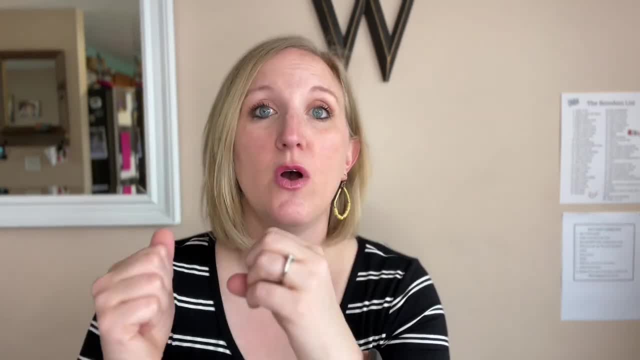 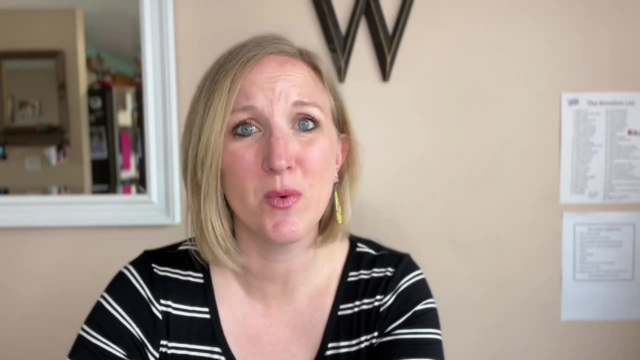 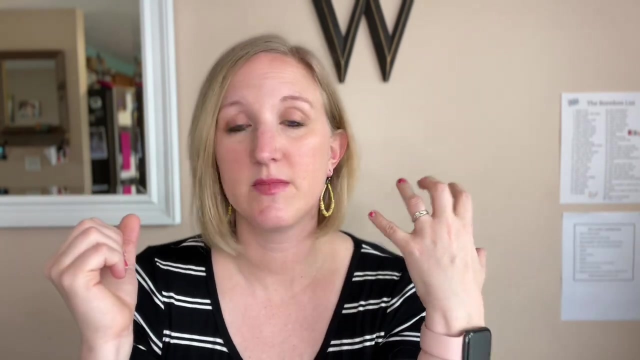 a workbook, but it's not a long drawn out workbook so it's not, you know, half an hour of the kids sitting at their workbook and doing it, especially at this age. you don't. you don't want that. so it's got a nice combination of both of those. it's got the hands-on mom helping games, things like that. 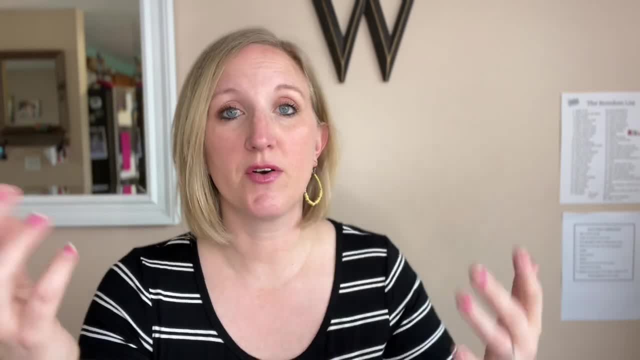 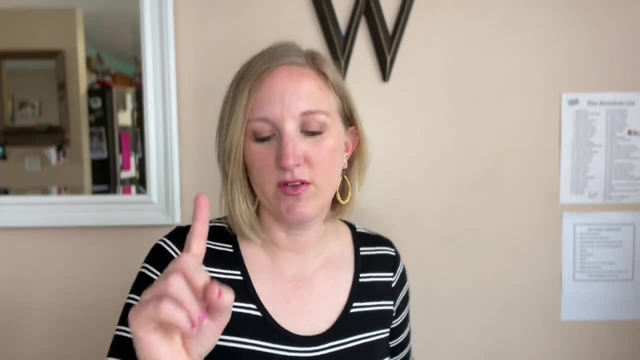 and then it has a little bit of independent practice doing the workbook on their own, and it's not too long. it is like just the like, oh, just like the sweet spot, like a nice little sweet spot for those things. for me, mom is still involved, yes, so it takes me about 10, maybe 15. 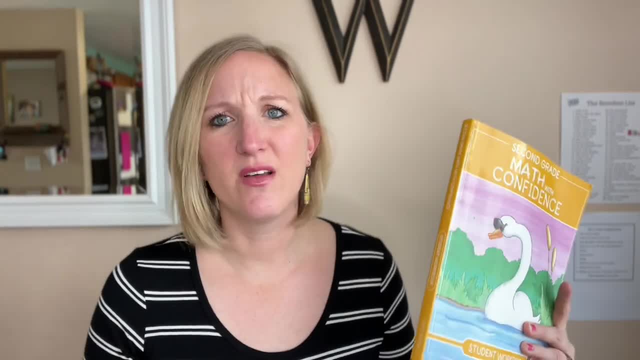 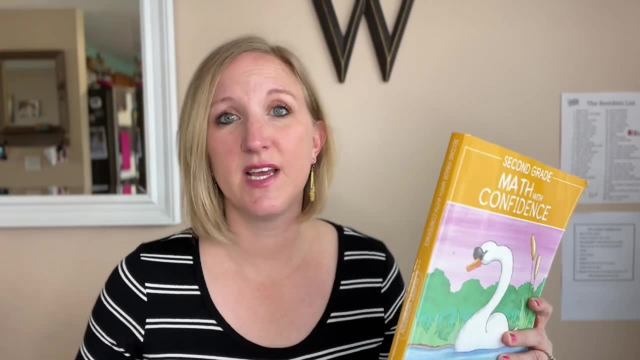 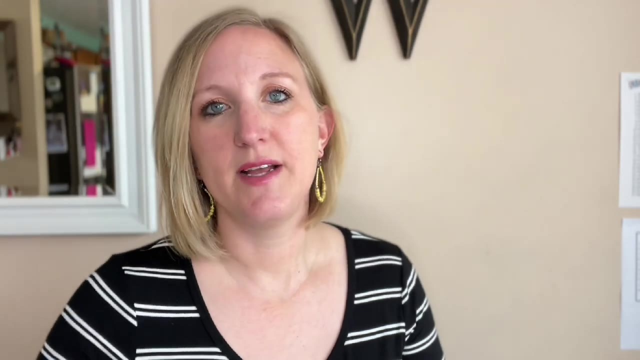 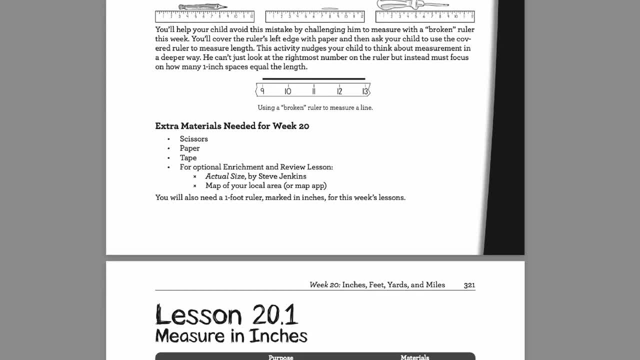 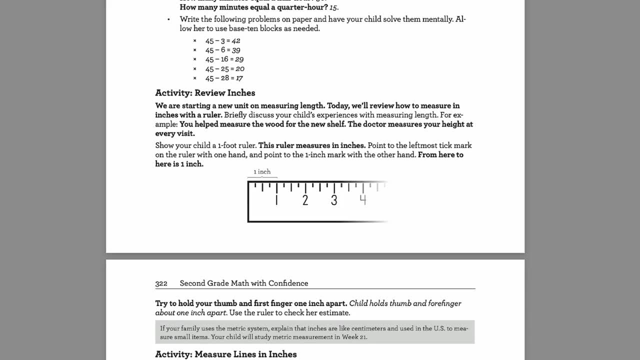 and it's short and sweet and to the point. it doesn't have long, long paragraphs for me to read to my son or long, long paragraphs for me to read to myself in order to know what to teach my kid. she like she gets in and she gets out. it's bullet pointed, it's to the point, it's clear, um. 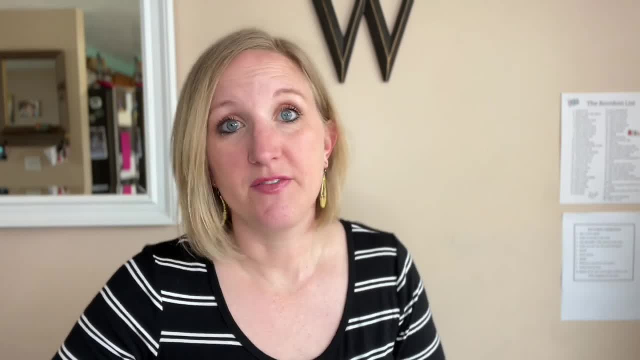 just well done. and, guys, i need to tell you i'm not an affiliate with this at all. i just love this math, so i will preach about it all day, every day. so i'm going to show you a little bit of my own math and then we're going to go through. 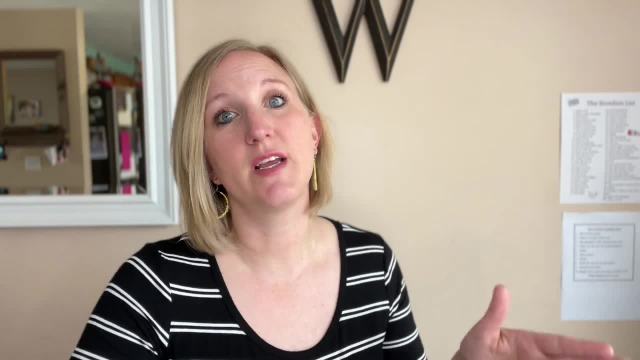 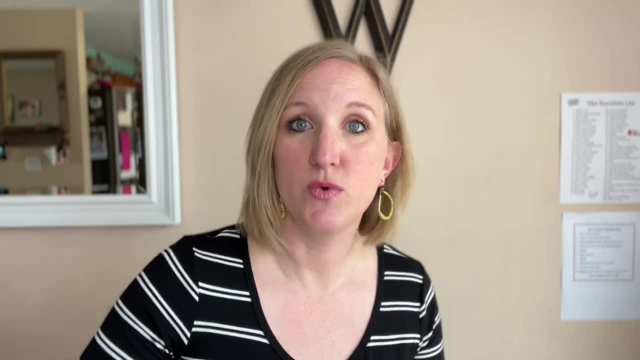 Right now they have available through second grade. Third grade Math with Confidence will be coming out for this summer, So if you have any third graders you can get the third grade version of this, just like my second grader will be moving into it. 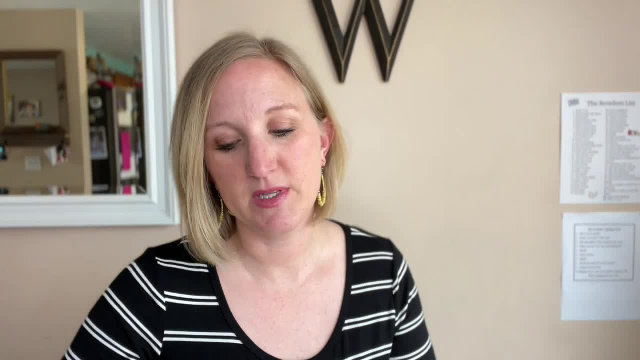 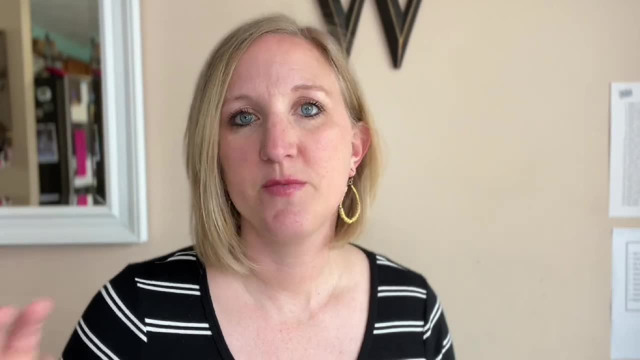 But maybe you have an upcoming second grader and you can definitely do that with this. If you are looking for anything higher level, it's not out yet. I'm currently in the pilot test group for the fourth grade- Math with Confidence, but that will be another year and a half. 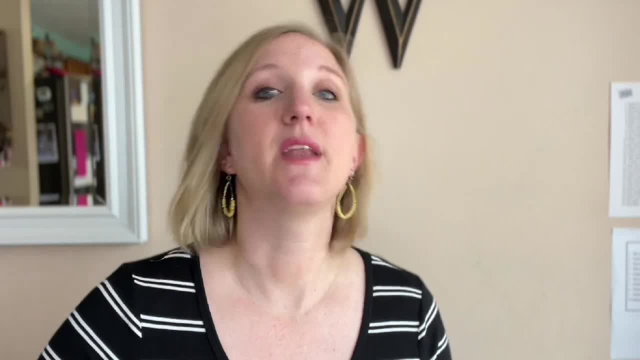 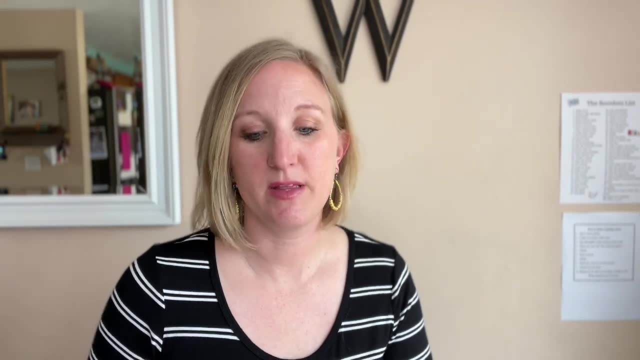 before that comes out, or two years. It'll be not this summer, but next summer is when fourth grade comes out, And then the following year, fifth and then eventually sixth. Oh, somebody asked me how do I organize my Math with Confidence. 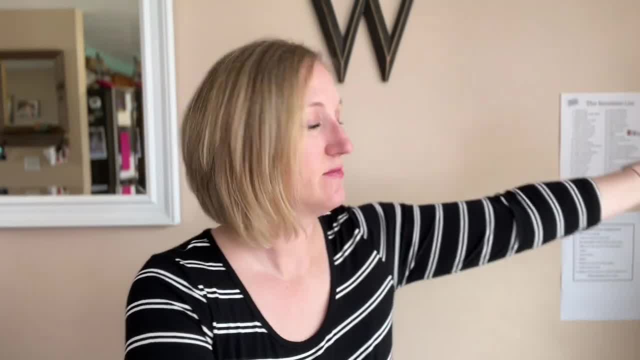 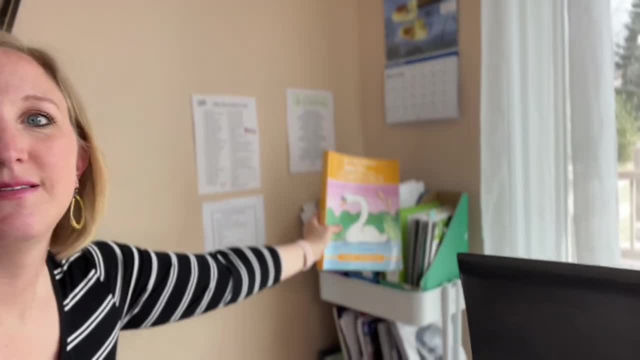 So this is my son's workbook and it stays in his shelf over here. This is where my kids keep their own books, Ta-da Okay. so it stays over there, and then he pulls it out when it's time for us to do our lessons. 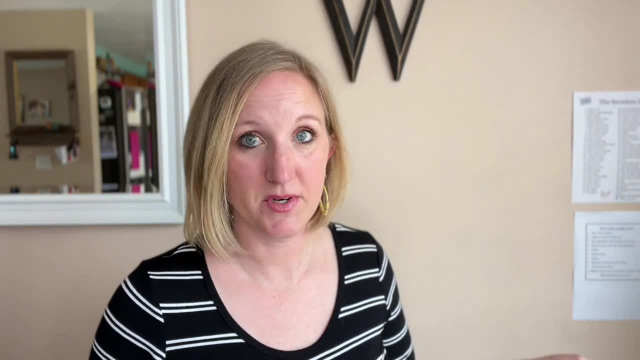 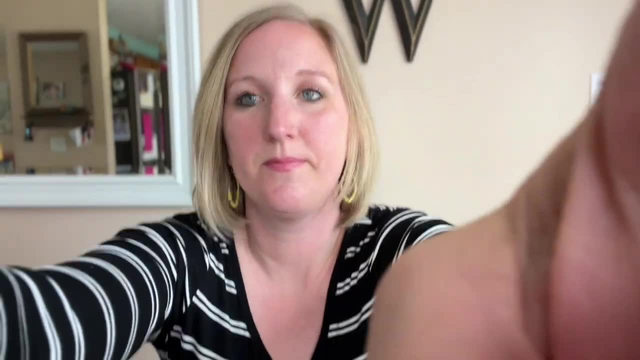 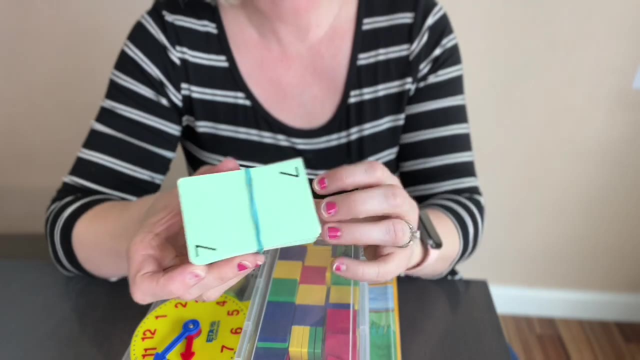 He also has all his like supplies down here. I'll show you. So I have this. I have this in a cart in our main dining room where we do our school. So I have our supplies that we need and that is a number, a deck of cards. 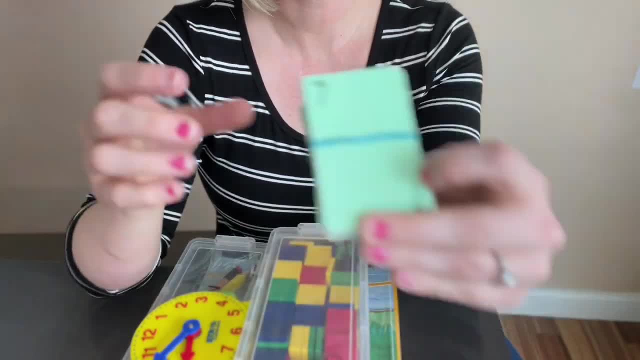 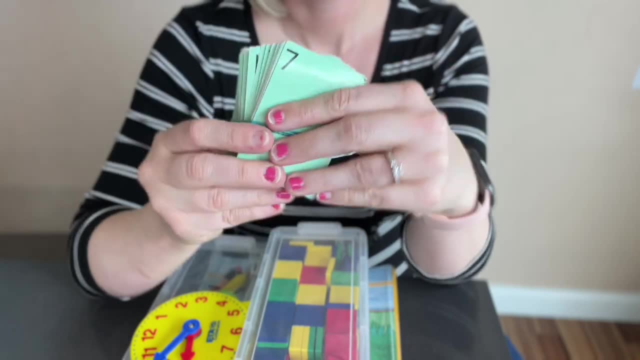 Kate Snow says you can use a regular deck of cards, but I use my Right Start Math deck of cards, So that came in real handy. So it's just the numbers, all the numbers, here. So you have your deck of cards. You're gonna use that for a lot of your games. 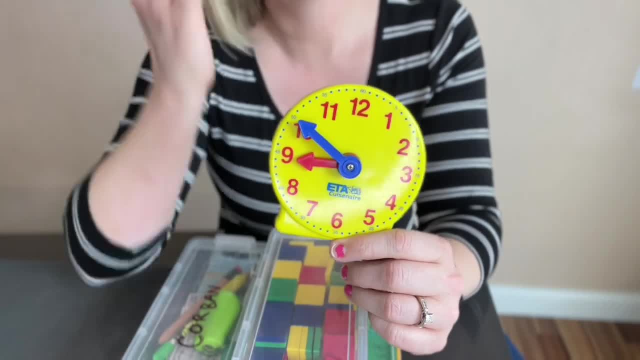 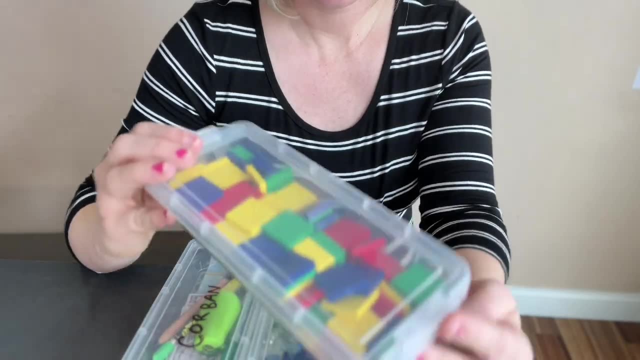 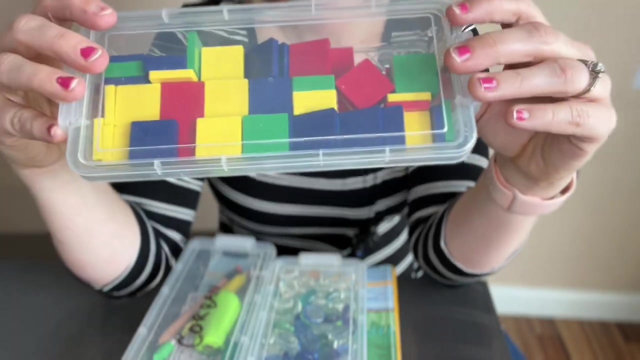 This: when we did our time unit, which we just finished, we needed the clock here and this came with my Right Start Math items as well. This also came with my Right Start Math items. I've used this for understanding measurement and understanding like addition, multiplication. 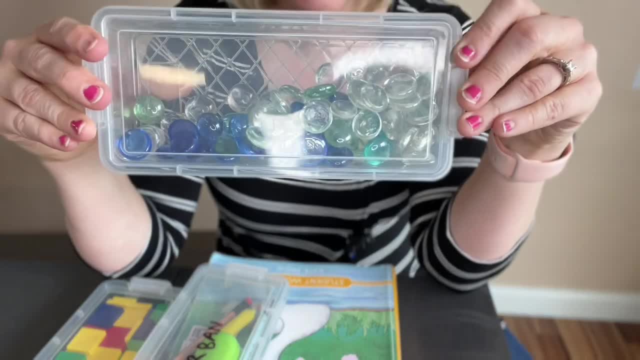 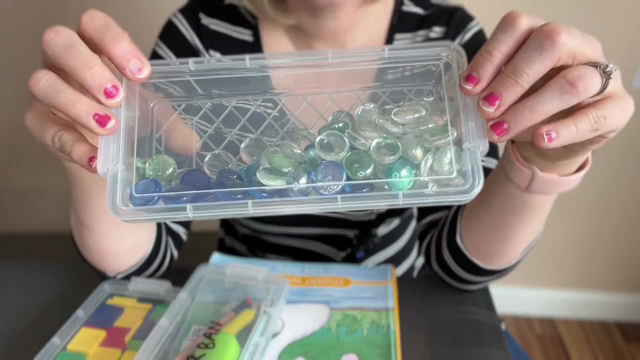 things like that. These are my counters. So you're supposed to have like little toys, like 6000.. tiny circular items and you can go buy some counters. but I got these at the dollar store and I already had them. They're the like glass beads and they stay in this little container. 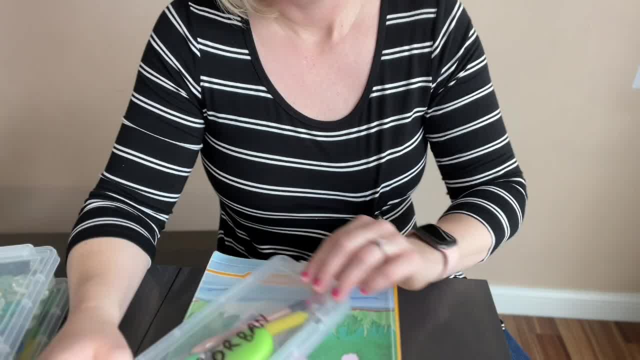 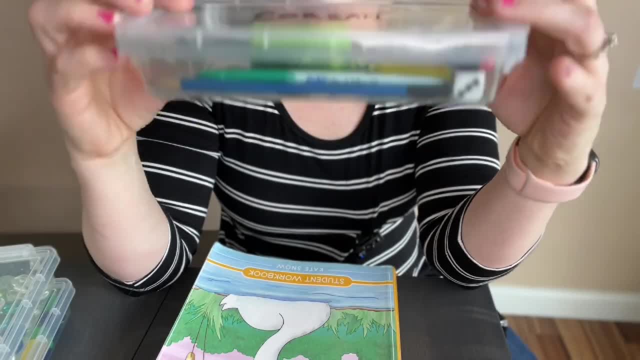 So we've pulled out for most of our games that we do, And then my son has all of whatever he needs in here. So we have a die, we have his pencils, we have some paper money and there is some like other money in there, like coins, markers and pencil sharpener that I keep in here. 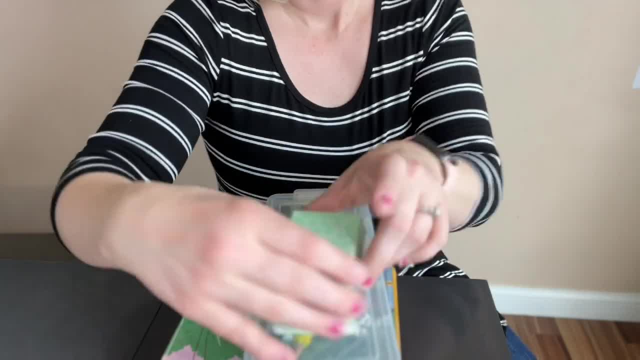 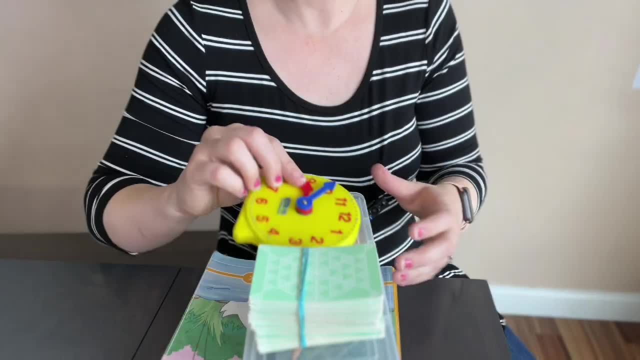 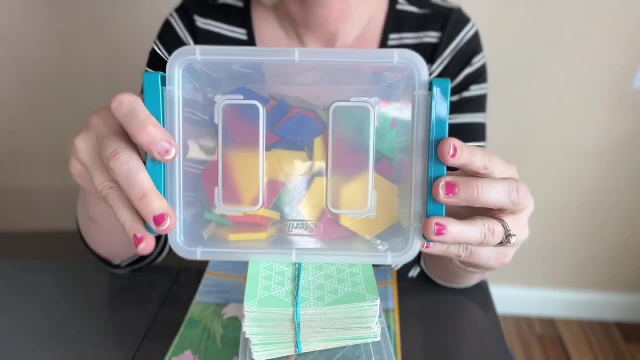 So that is all my supplies. I don't know. I can probably fit this in a bin somewhere, but it just stays out because I use it so frequently. And then we've got, and then the clock there, So these all fit on my shelf over here. Yeah, these ones, these are the other ones that I've used, The 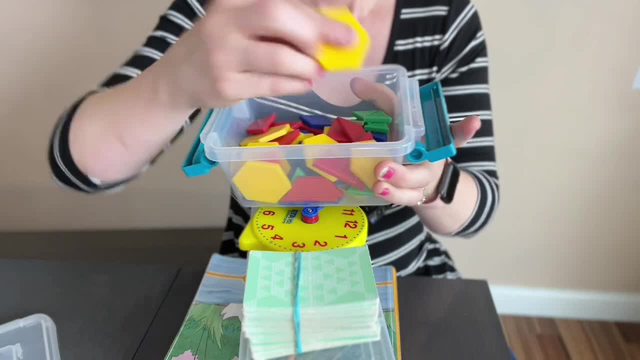 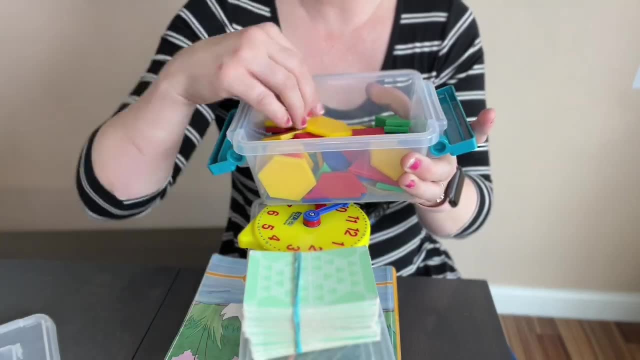 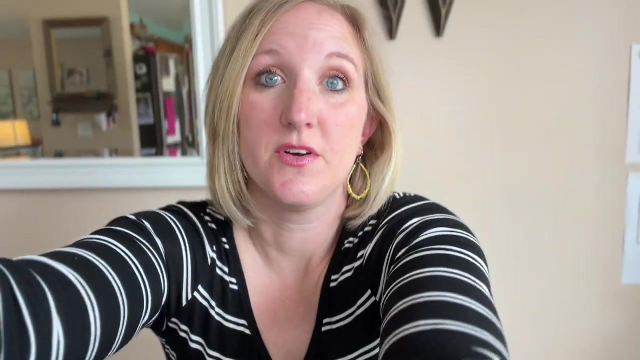 pattern blocks, the shapes. So you use these for sometimes lessons And I got these a long time ago. I've had them for all my kids, But those stay in that bin and they all stay on the bottom shelf right over there where my math stuff is, So it just stays right there. Want to look at it? Do you want to look? 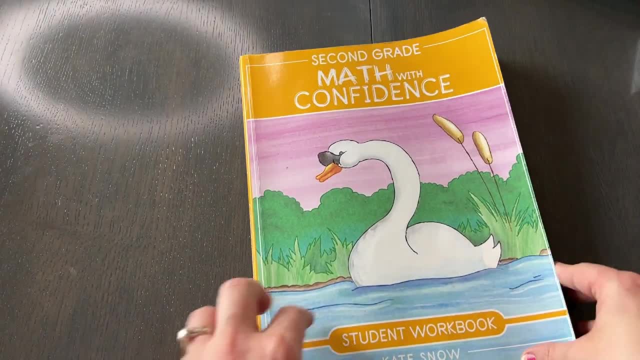 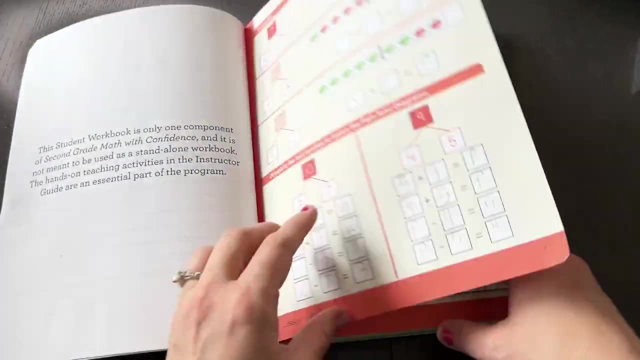 inside. All right, So let's look inside the workbook. This is the student workbook, So for each lesson they have two pages, So just front and back and that's it. So like this one is lesson 1.4 and lesson 1.4 and that's it Usually on the front. they can do it by hand, but they can't do. 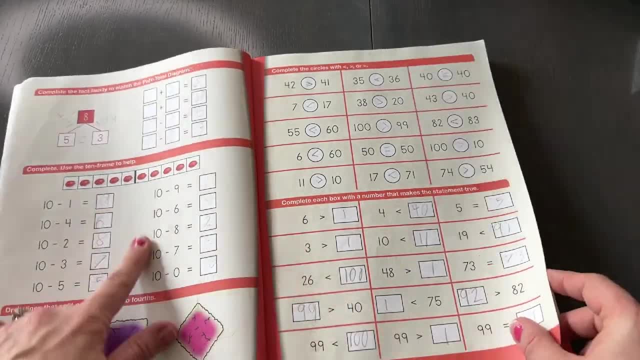 it by hand. So they can't do it by hand. So they can't do it by hand. So they can't do it by hand. But if they need help, they can always ask. But the back page is usually review, So the first page. 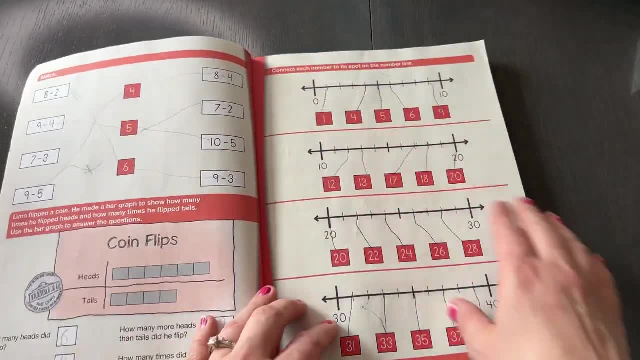 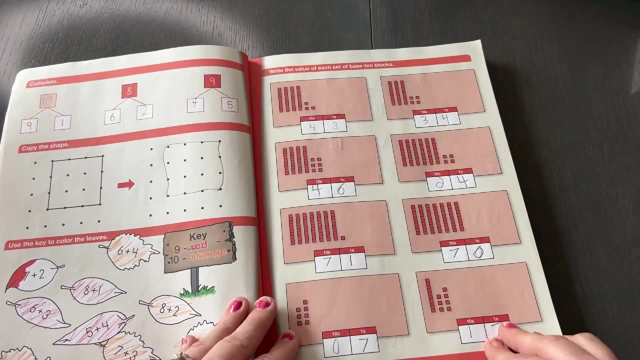 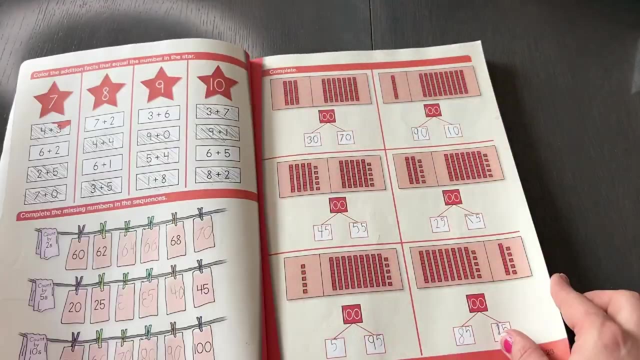 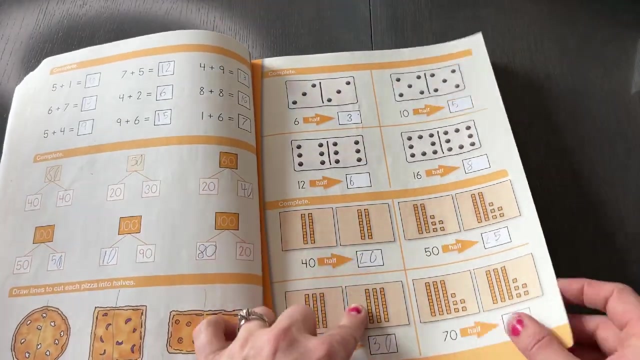 is practice of the lesson that you just did. Then the back page is a review of something you've done in the past. So here we've got learning. What is this? What are they called The base 10.. There it is Base 10 blocks there, And then more review And then it moves into 6.1. So learning more. 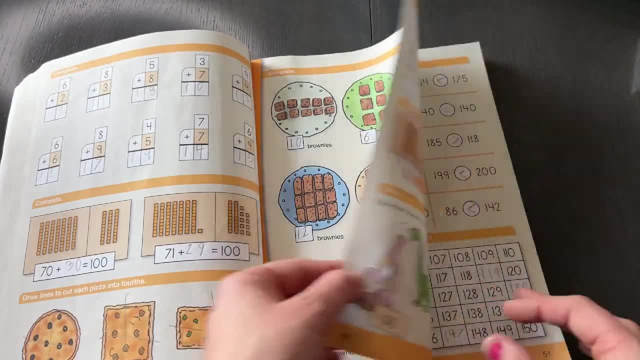 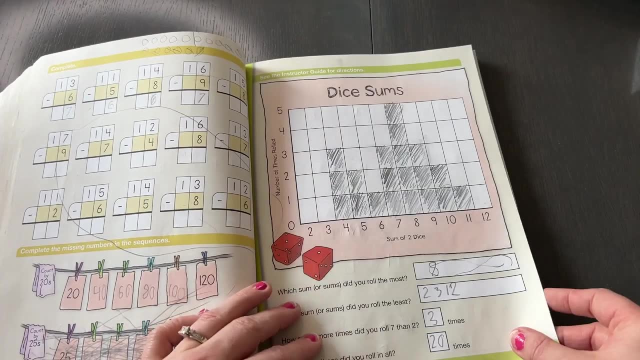 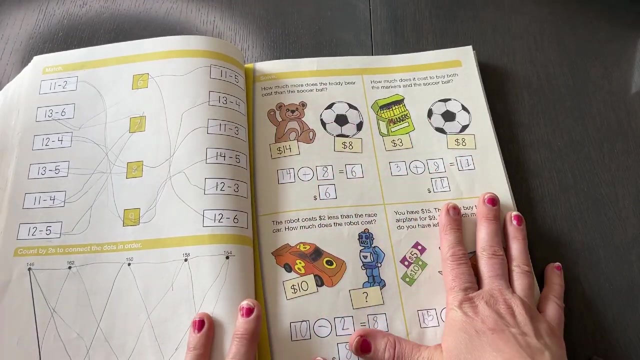 and more. And then we have subtraction, addition, looking for patterns greater than less than, And then we had a graphing unit recently, And then we have so again, it's not overwhelming. So look at this: When she gives you word problems, it's only four to do, So it's not like you only have just. 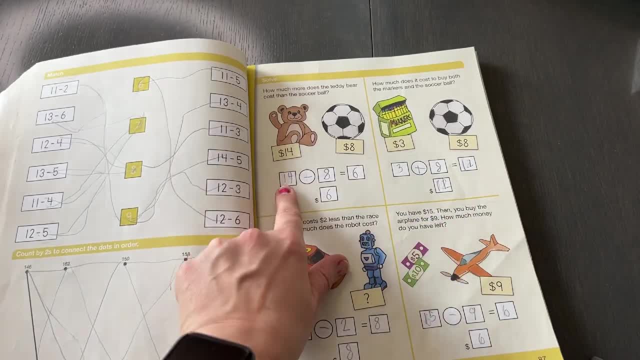 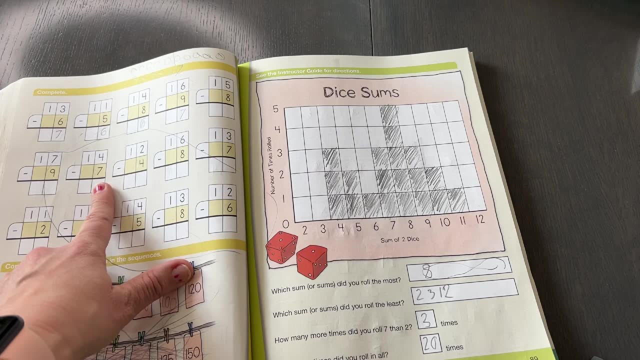 words on the page And I love how clean and simple it is And I love she gives you little spaces to write the numbers in. And then we have subtraction, addition, looking for patterns greater than, less than, And then a little bit of practice here, And sometimes we just do these orally or he will. 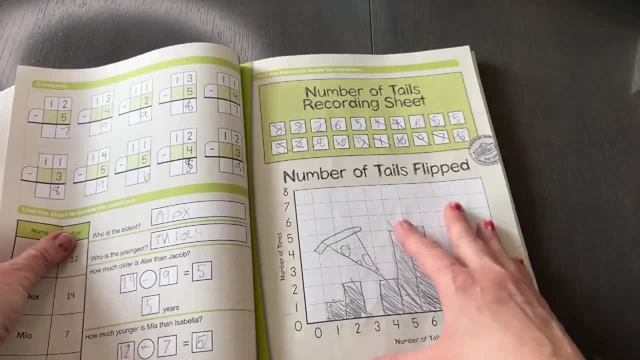 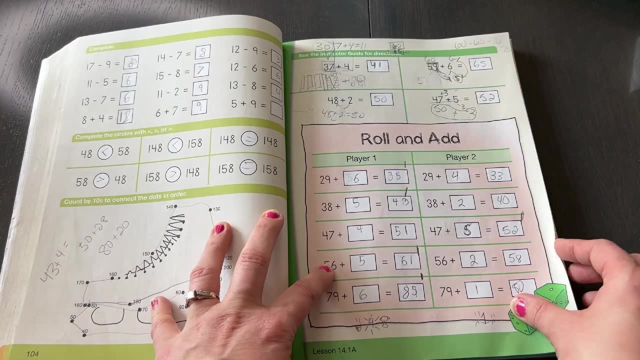 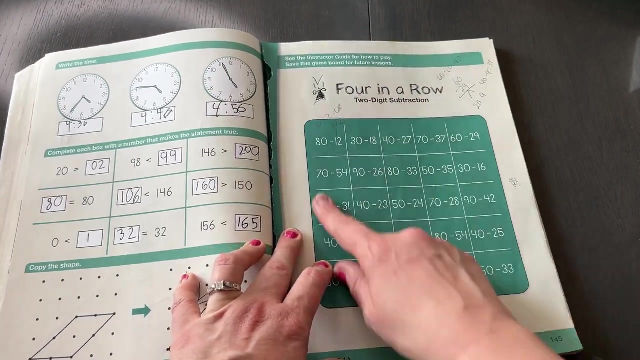 say it and then I will write it down instead of him writing it down every time. Here's an example. I probably wrote these, I think. So we play some games that we do together. So you needed a dice for this game And then we had like four in a row, two digit subtraction. We needed our counters for. 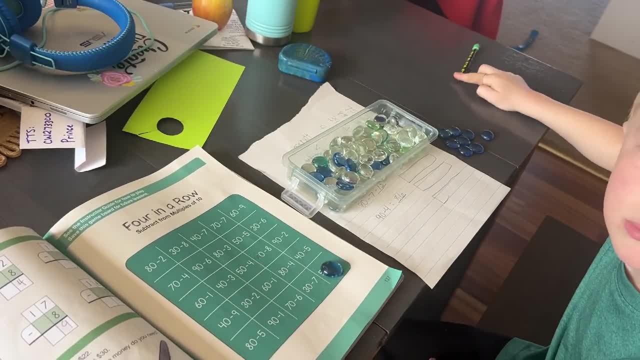 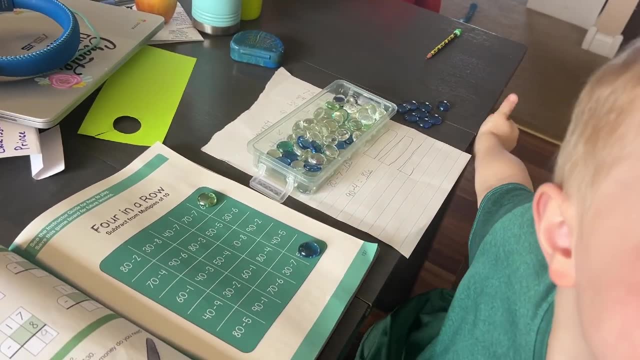 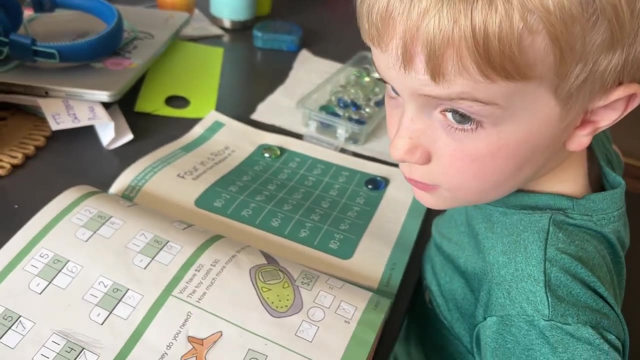 this, It's 47.. Okay, I'm going to go over here. 60. We need our counters, So 0-9 would be 61.. Right, Almost said 59.. I didn't do my math, right, Pick one. 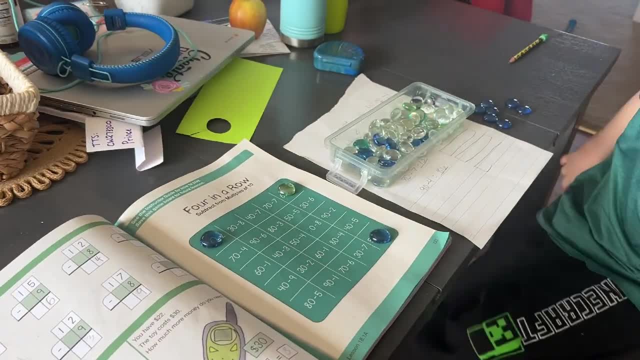 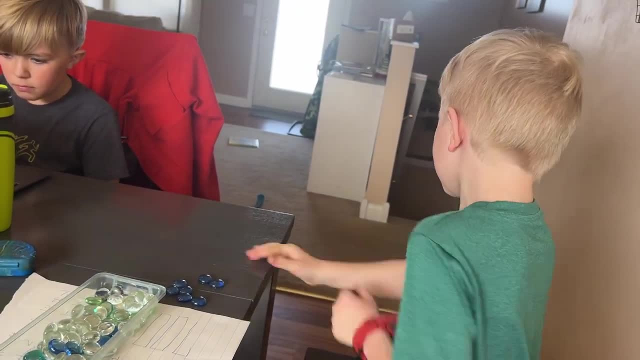 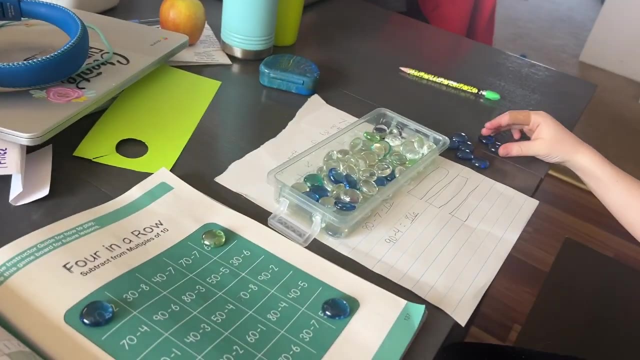 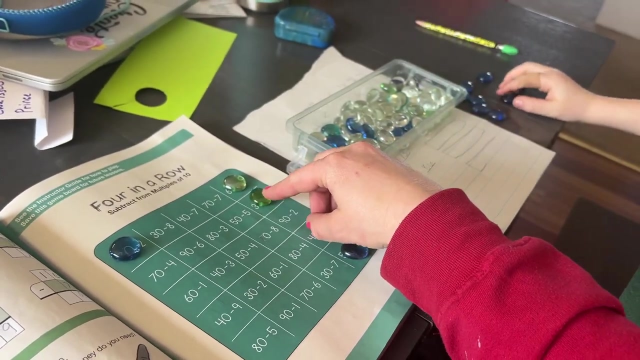 AB-2: equals, equals, equals, equals, equals, equals 78.. 78.. Good job. Okay, Now my turn. so our goal here is: try to get four in a row. I'm going to go here: 30 minus six is going to be 24.. 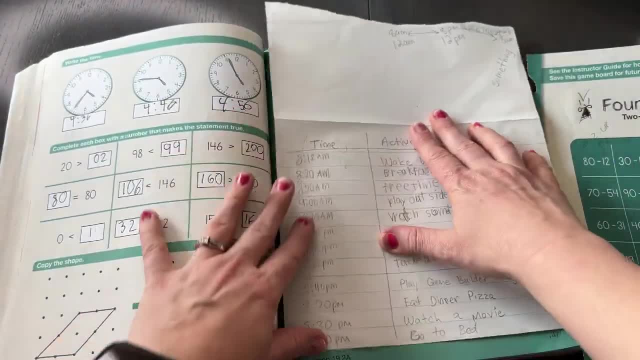 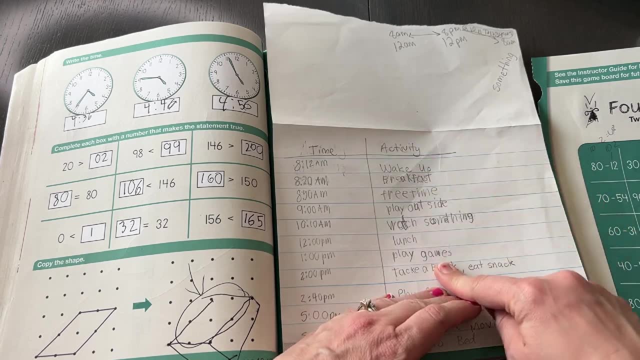 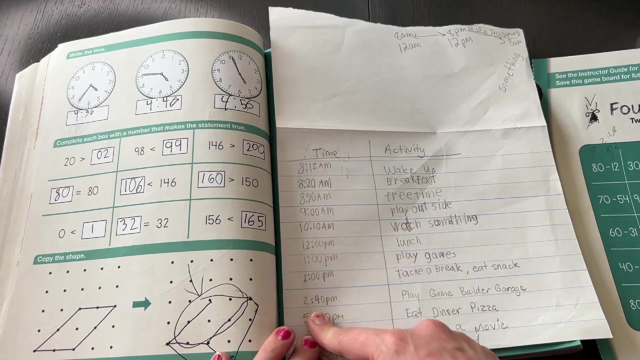 One of the lessons for time we just did recently was him make. he wrote this all the way up until here. He wrote this whole thing. I was very impressed, Um, and then I had to write the end of it. but we we were looking at like AM and PM and we're looking at time moving throughout the. 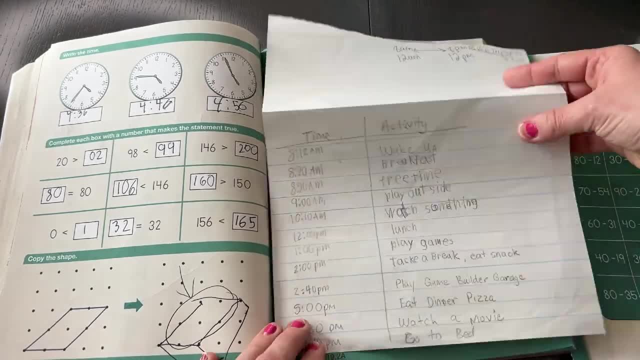 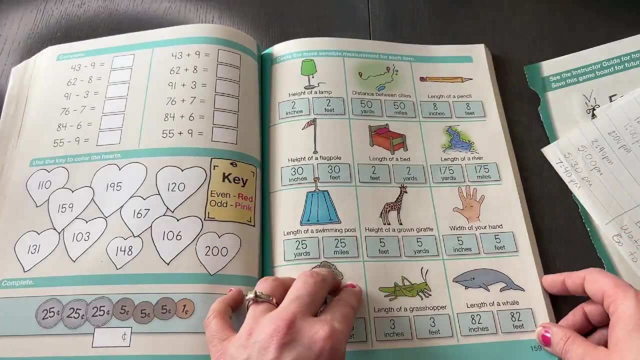 day and then what he does throughout the day. So that was a neat, just simple little activity. And then we have some things here later in the year that we haven't gotten to yet that you can just take a peek at. So I love this workbook. Look how simple it is. Here's another. 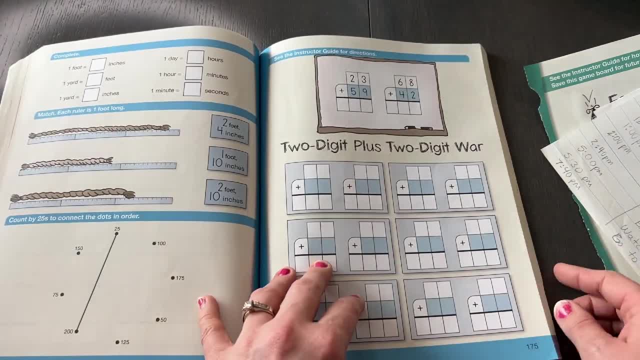 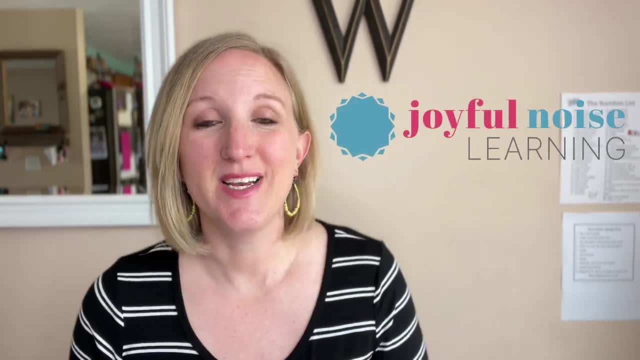 game that you'll be playing: a two digit, two digit plus two digit war. So if you want to know a little bit more about me, welcome to joyful noise learning. here I like to talk about Charlotte Mason inspired homeschool, biblically based curriculum. 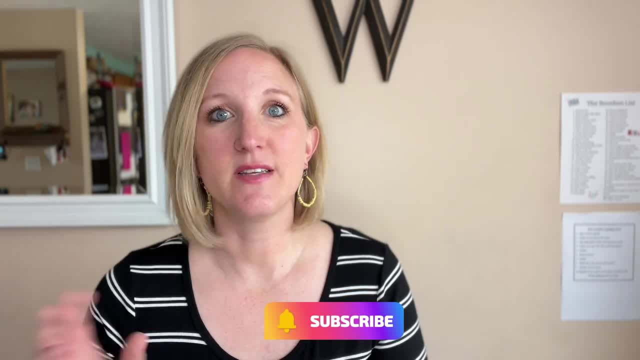 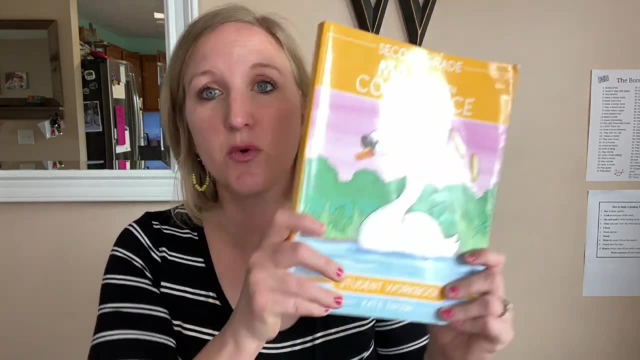 and uh, encouraging the scattered brain, easily distracted homeschool mom. As far as the instructor's guide, I don't have. I only have a digital copy of the instructor's guide, So I don't have one to flip through for you If you've seen the flip through of the kindergarten. 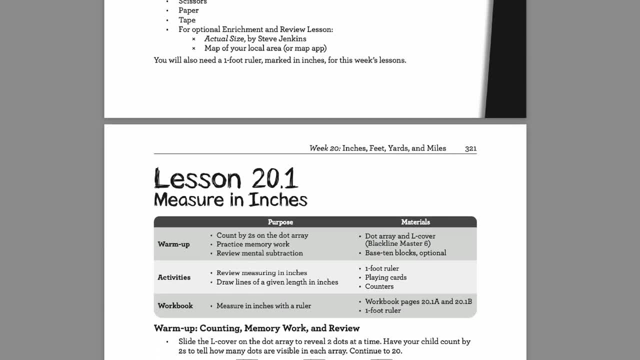 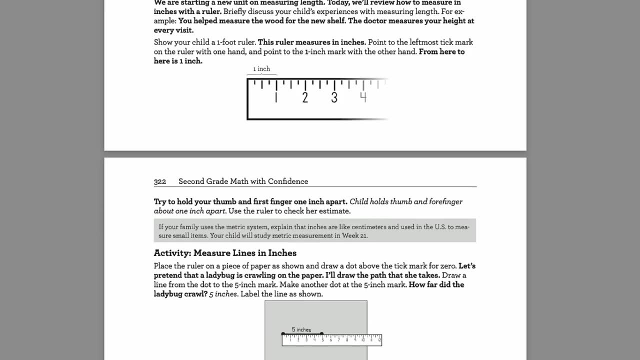 math of confidence. it looks very similar. It's laid out the same, uh, simple to follow, Like I said earlier, and it has instructions there for the games that you need to do. You start out with a warmup and it's usually just asking a few memory work questions Like. 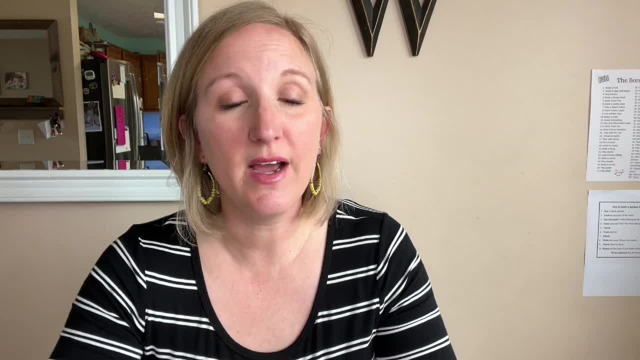 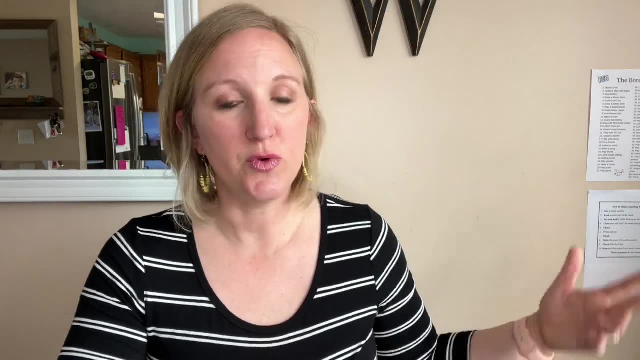 what do you call 12 o'clock at night, Like when you're asleep and it's it's- another word is midnight. What do you call 12 o'clock during the day? at lunch It's noon. Uh, then you have him. 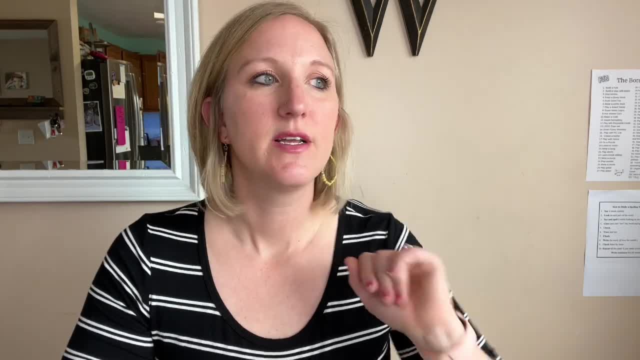 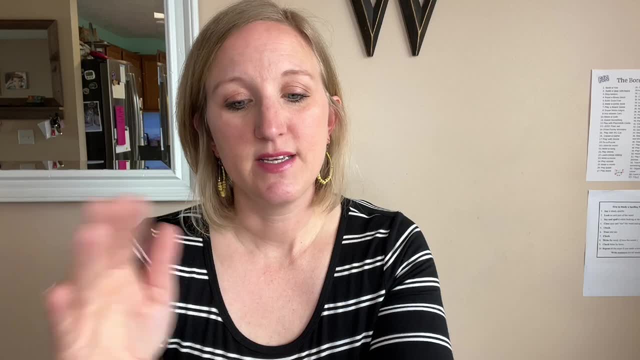 practice counting by tens or counting by fifteens or counting by twenties, you know, like those uh, like those kinds of warmups, uh, that you do quickly and briefly at the beginning of the lesson. Then it goes into the explanation of what you're learning and then you practice it together And 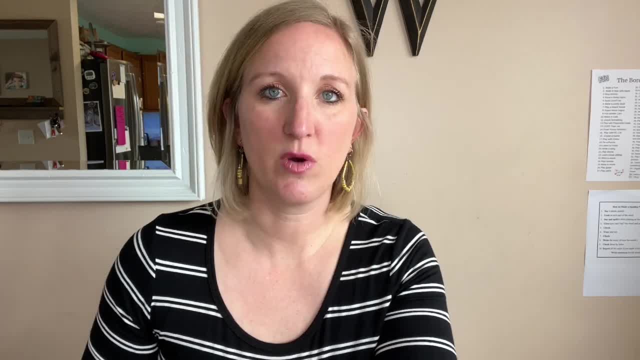 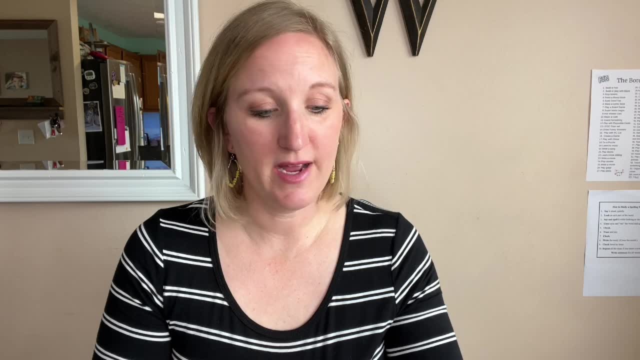 then you play a game to practice it, And then you practice it together, And then you practice it together, And then he does his workbook or she or your daughter does her workbook, And that is it. Like I said, she streamlined everything I loved and wanted in a math curriculum And it. 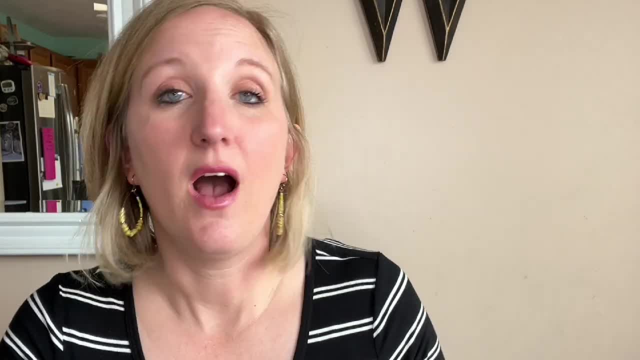 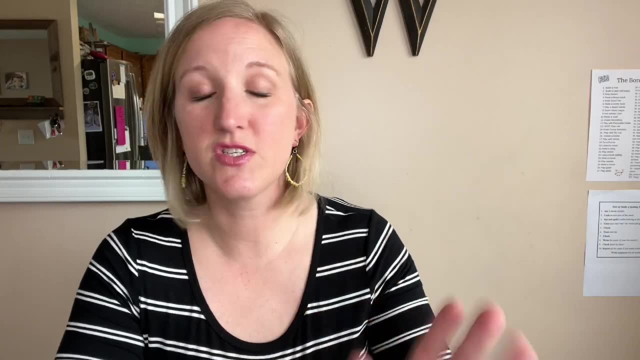 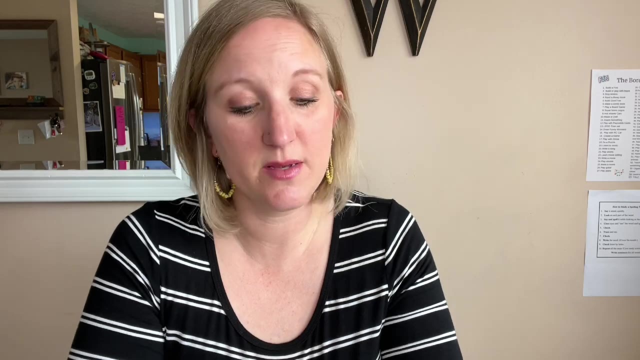 is all there. Some people asked if it was enough and I very dang well think it is. I think it is enough And my kids are. my kids are doing so well with math. Part of that may have to do with my son's personality: He is bent towards math. It's one of his favorite subjects, He says.